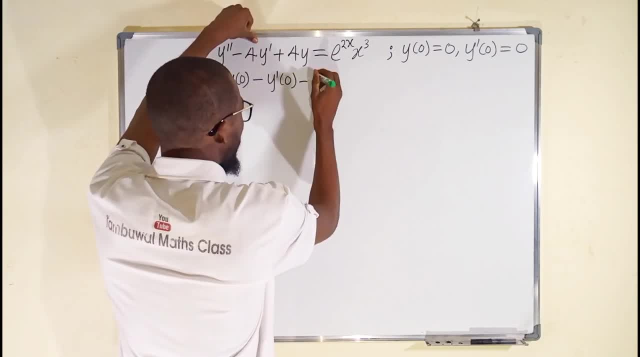 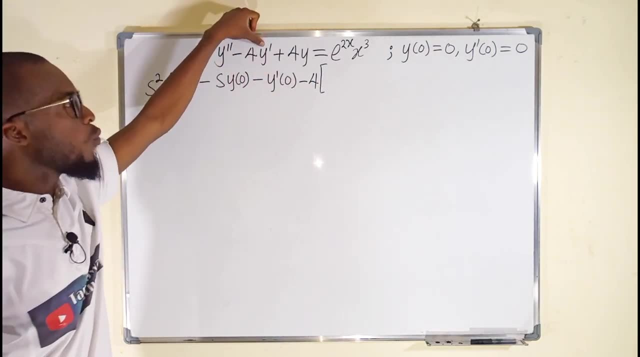 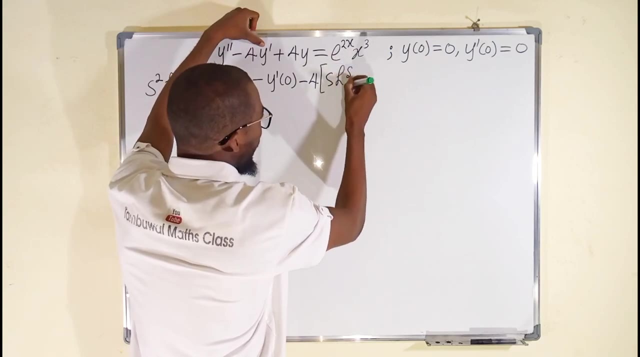 negative 4.. Then we take the Laplace transform of y prime. Alright, We have factored out negative 4.. The Laplace transform of y prime will be s, because the order is 1 multiplied by the Laplace transform of y. Then you subtract The. 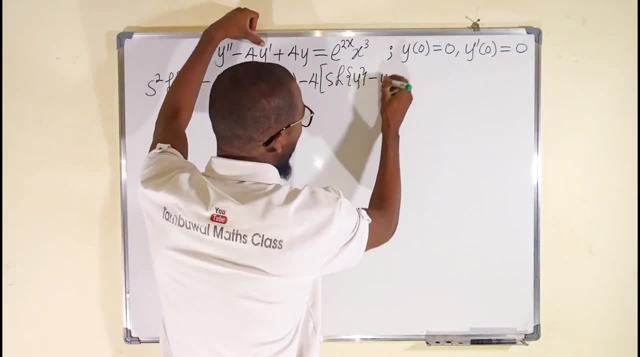 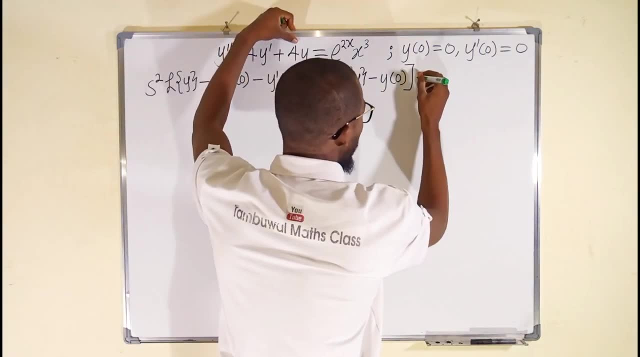 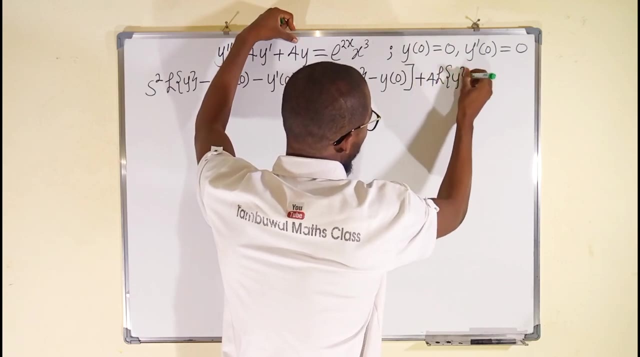 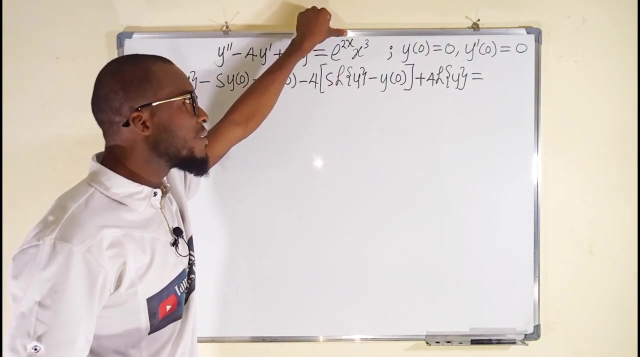 power of s will reduce by 1.. We just have y of 0. Moving on, We have 4 outside multiplied by the Laplace transform of y, and to the right hand side we have the Laplace transform of e to the 2x then multiplied. 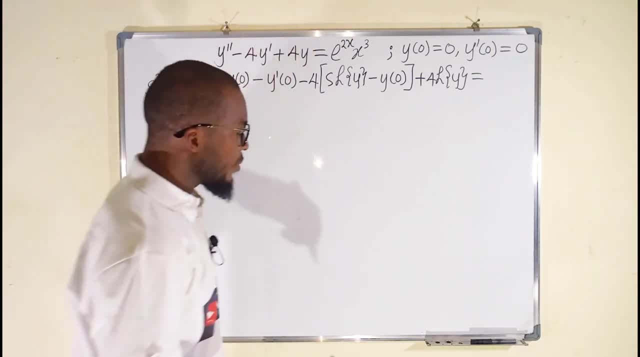 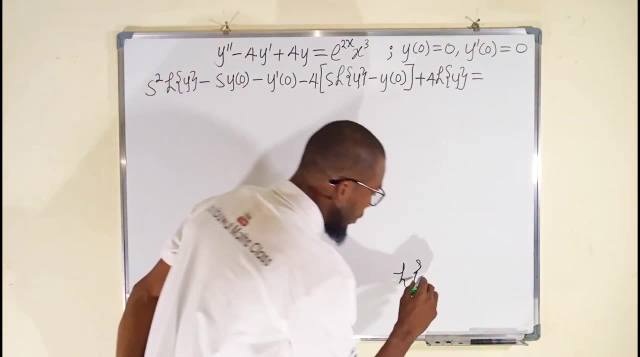 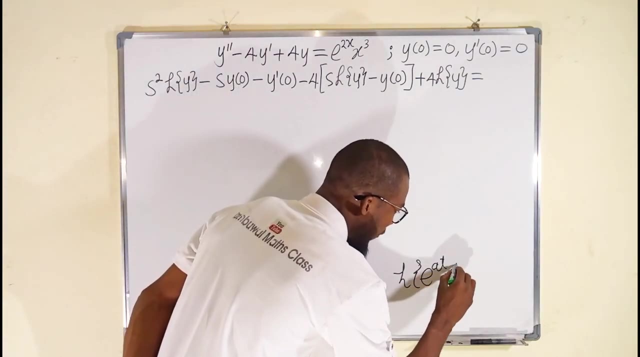 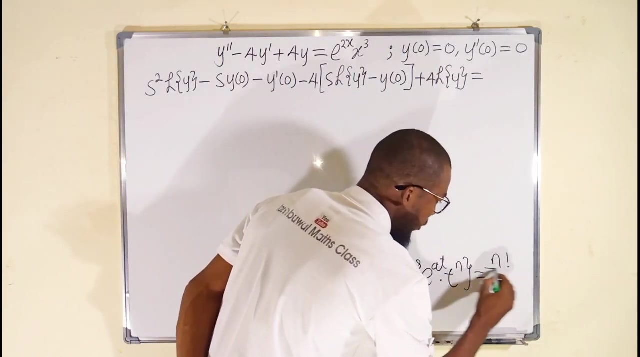 by x to the power of 3.. Okay, Let me remind you of something. Remember: if we have the Laplace transform of e to the at, multiplied by t to the power of n, This is equal to n factorial divided by s minus a, which is the coefficient of t. here, Male to. 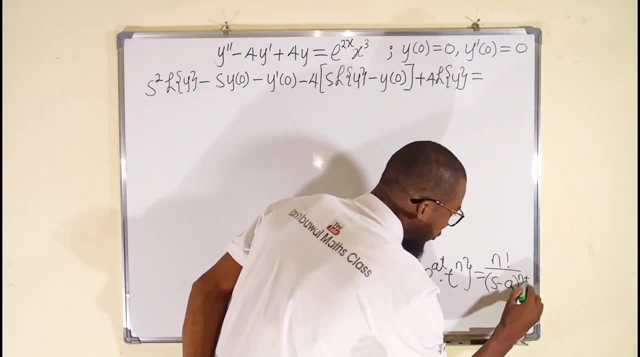 the power of n plus 1.. how do you do that? We always dia 않bags, because we always have e to the power of n at, But instead you no end up having the last one. So let me show you how to do that. So first you sidetrack and then delivery that to the 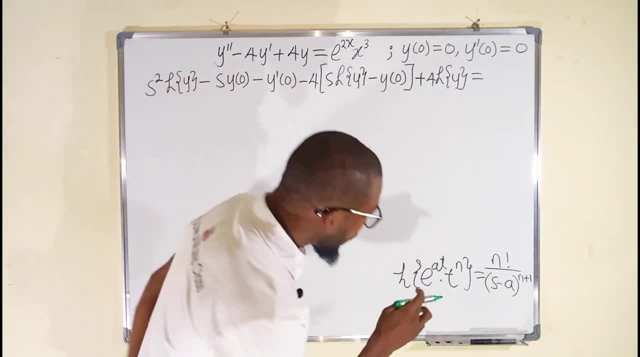 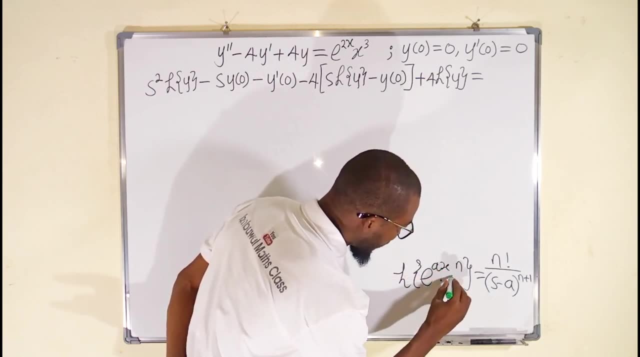 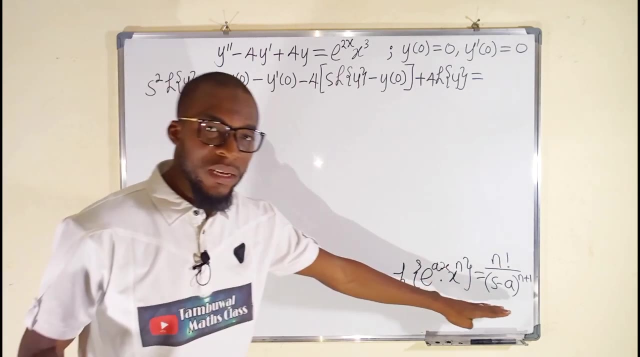 But remember, our function is in term of x, So we can just replace this and this by x, So this becomes ax and this becomes x to the power of n. So let us relate this and this so that we can get our Laplace transform. 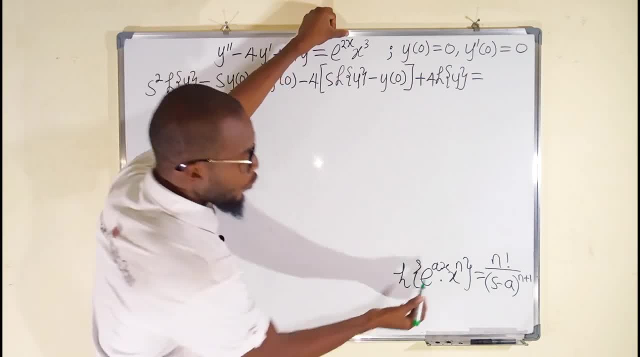 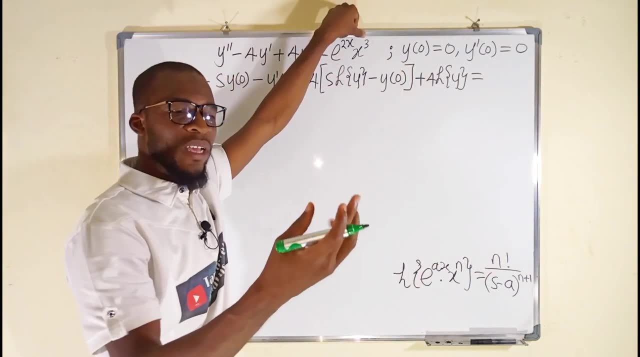 Therefore, the Laplace transform of e to the 2x, where our a here is 2 and our n here is equal to 3.. We have 3 factorial, which is the same thing as 3, multiplied by 2,, multiplied by 1, which is the same thing as 6.. 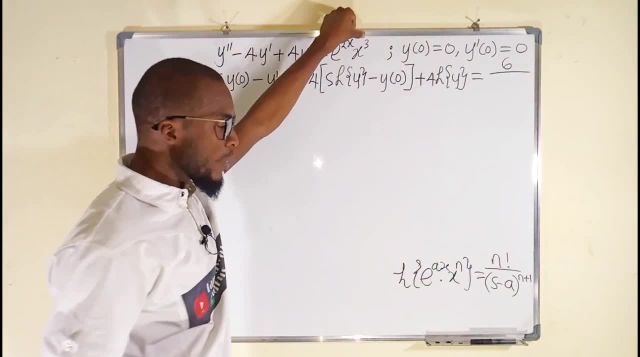 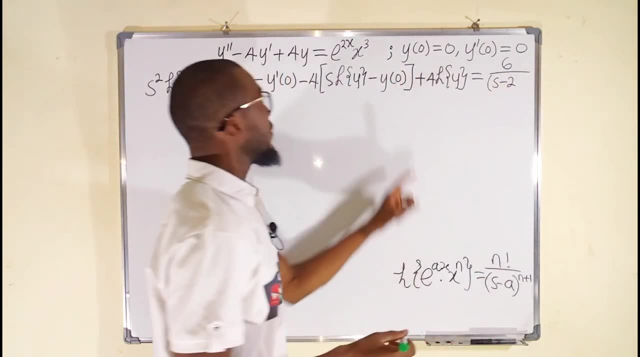 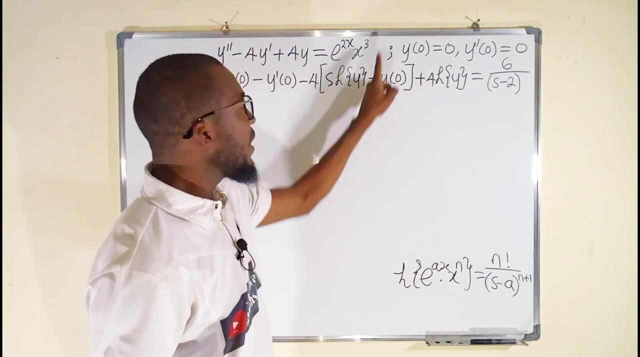 So we have 6 here. divided by s minus a, We have s minus 2, because a is equal to 2 here raised to the power of n plus 1.. Our n is 3 plus 1, equal to 4.. 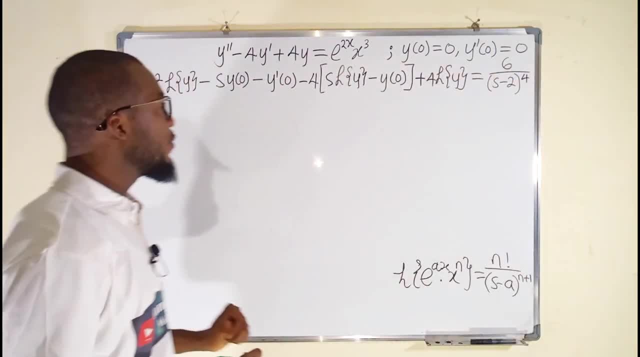 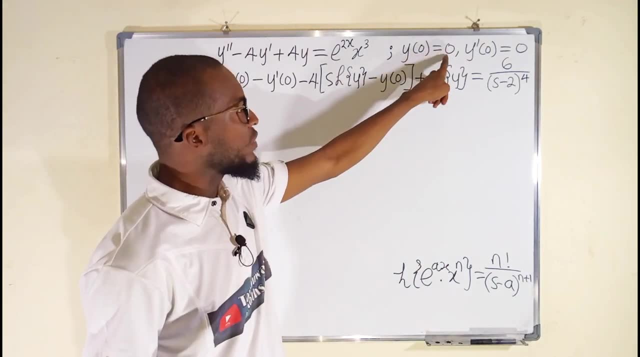 So we have 4 here. This is still usual. Let's continue. But we can just substitute our initial conditions here You can see: y of 0 is equal to 0.. y prime of 0 is also equal to 0. 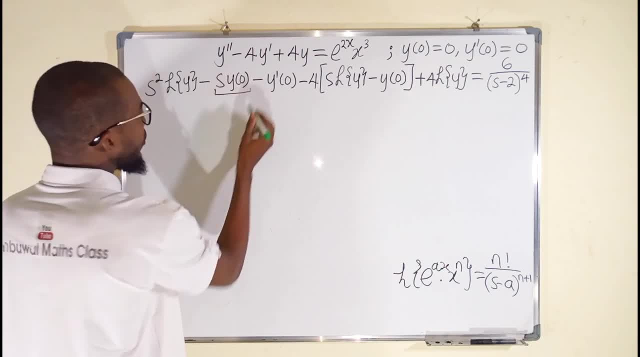 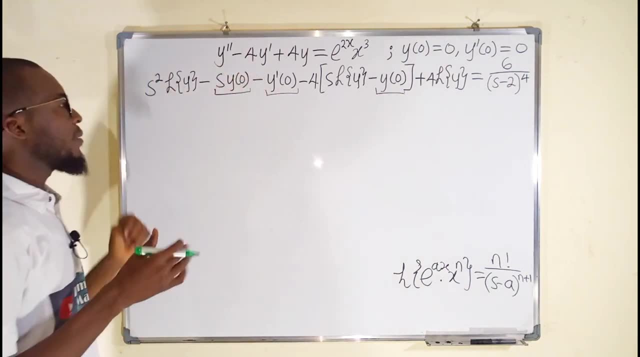 So let me mark them. We have this equal to 0.. We have also this equal to 0. We have this equal to 0.. I want to neglect them, So the only terms we have is this: Then we distribute this negative 4 over here. 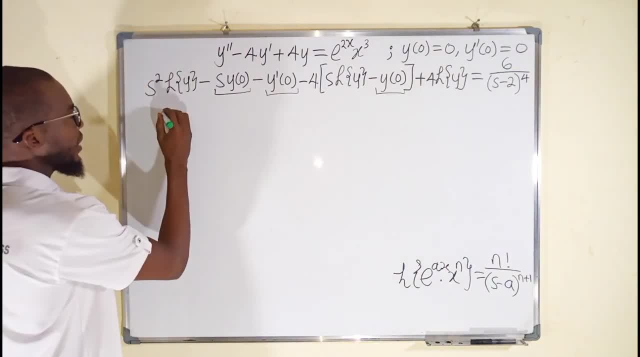 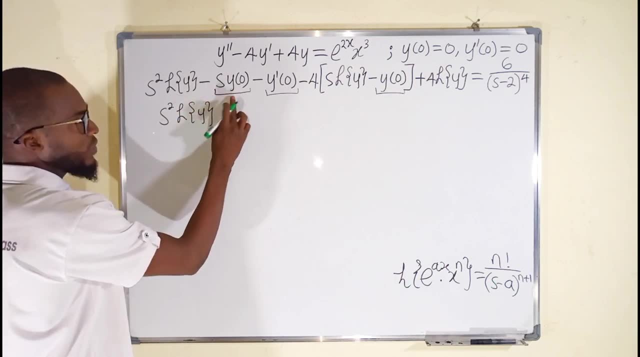 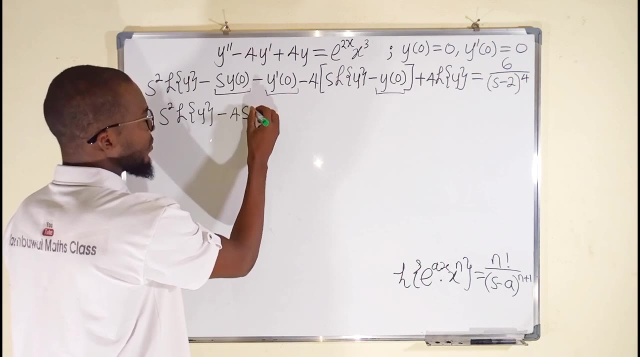 And this one and the last one. Here we have s power 2: Laplace transform of y. This is 0.. This is 0.. Then, minus 4 times this, We have minus 4.. 4s multiplied by the Laplace transform of y. 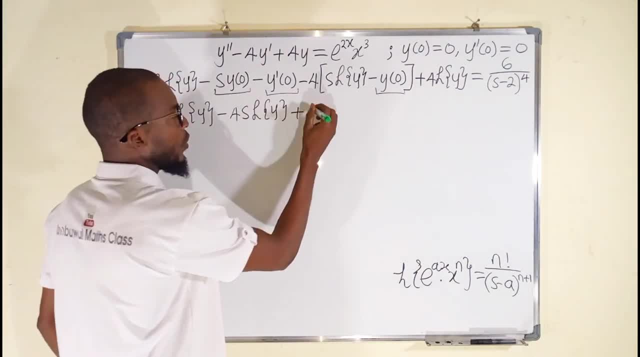 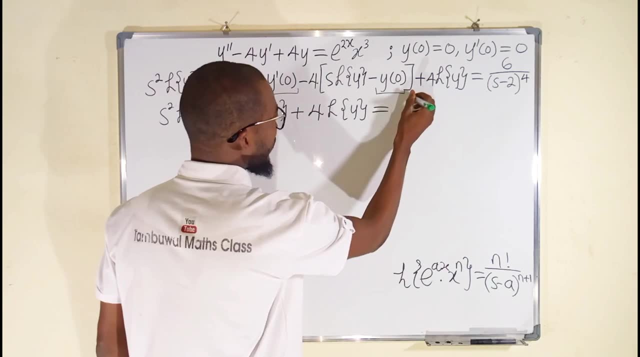 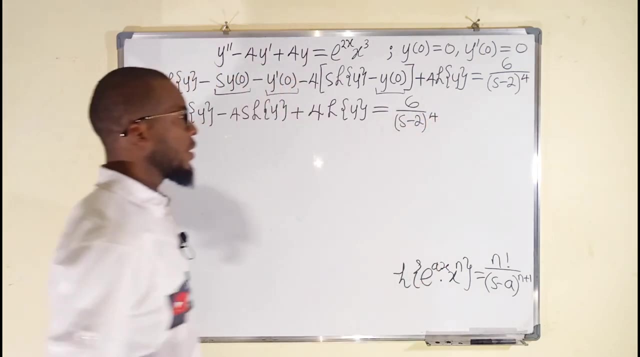 This is 0. Then we have plus 4 multiplied by the Laplace transform of y, y. And to the right Hand side, We have 6 divided by s minus 2 to the power of 4.. Okay, Now let us factor out Laplace transform of y. 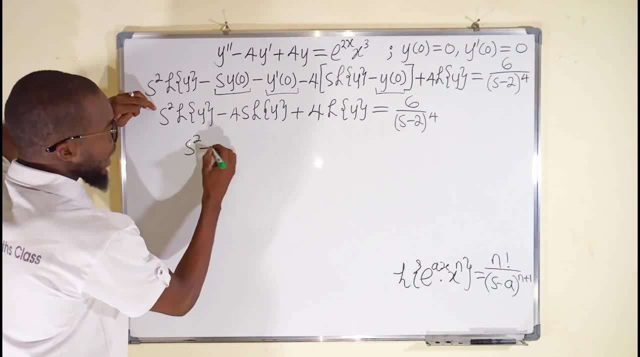 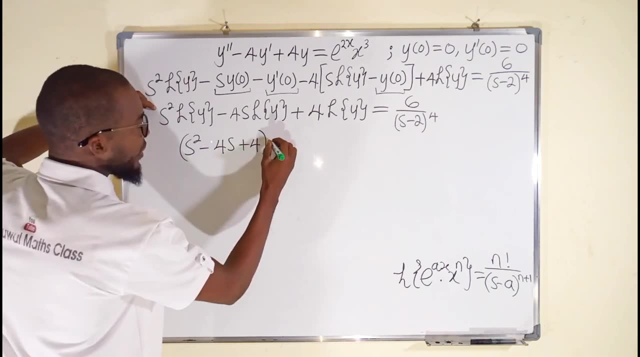 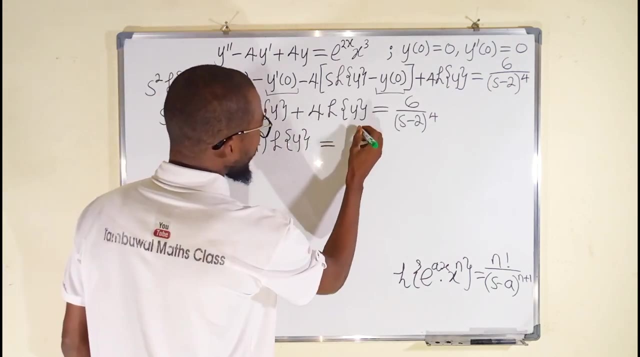 We have s power 2 minus 4s, then plus 4.. All of this multiplied by the Laplace transform of y And to the right Hand side, We have 6, divided by s minus 2, to the power of 4.. 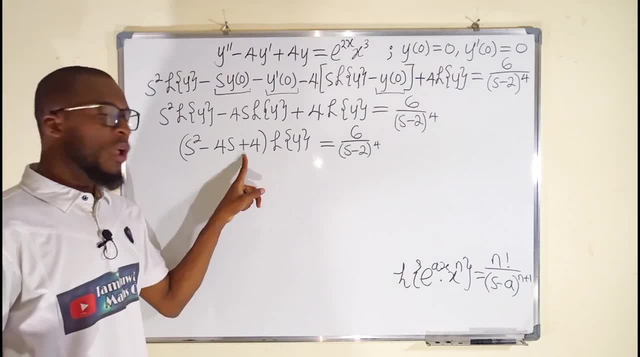 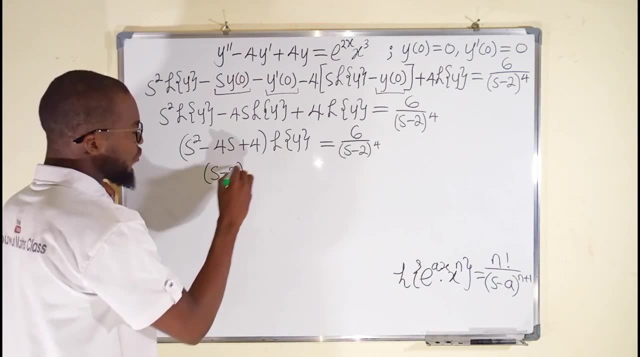 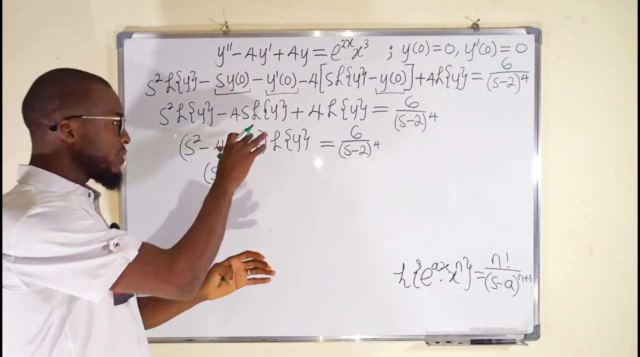 We are moving. This is a perfect square. quadratic trinomial, Which is the same thing as s minus 2, to the power of 2.. Remember, half of 4 negative is negative. 2 squared is 4.. This means that this is a perfect square. 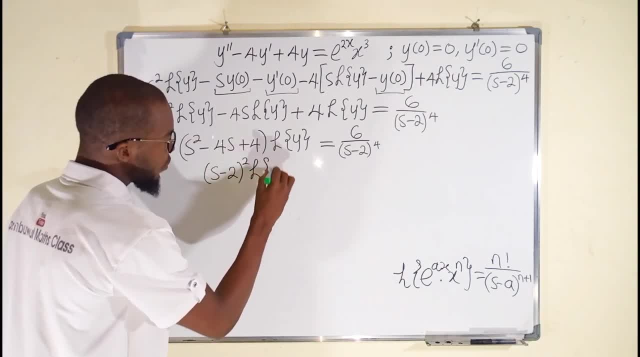 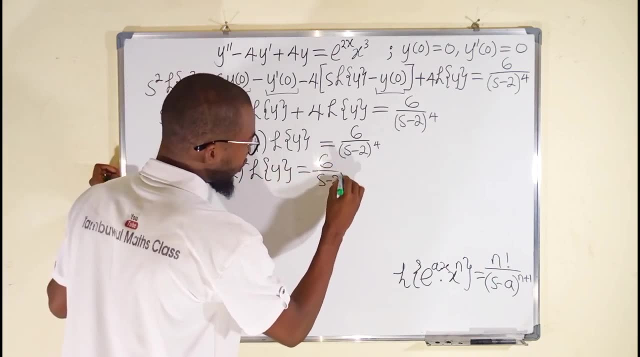 Multiply by the Laplace transform of y, All of this, And this is equal to 6, divided by s minus 2, to the power of 4.. And this is equal to 6 divided by s minus 2, to the power of 4.. 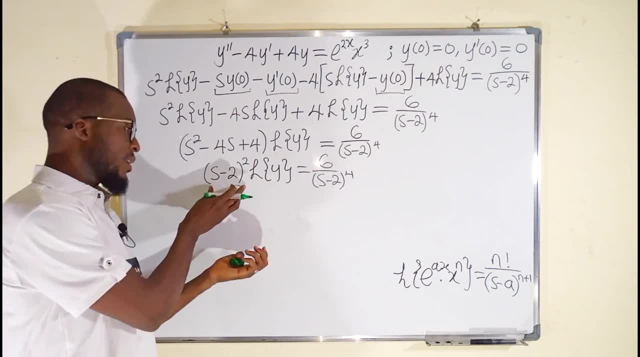 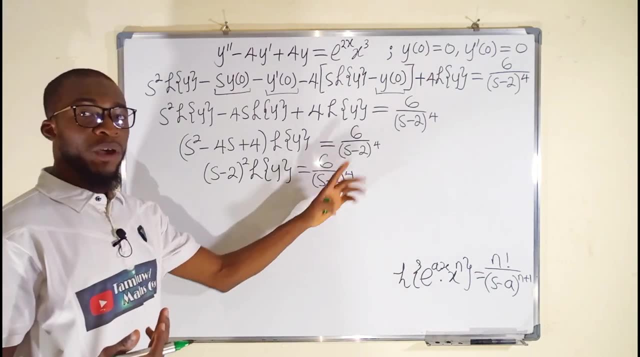 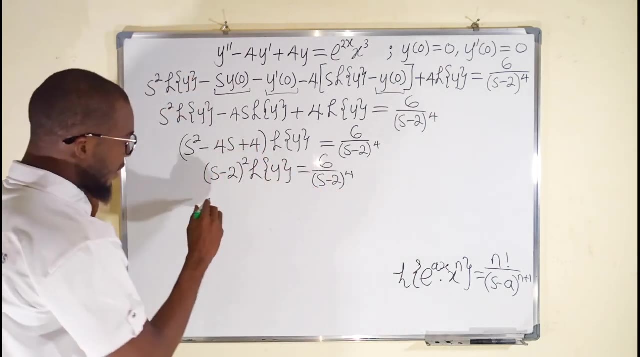 Let us bring Laplace, transform to the left and take what I mean here. Let us divide both sides by s minus 2 to the power of 2.. Already, this is s minus 2 to the power of 4.. If you divide, it will multiply the denominator. we have powers 2 plus 4, equal to 6.. 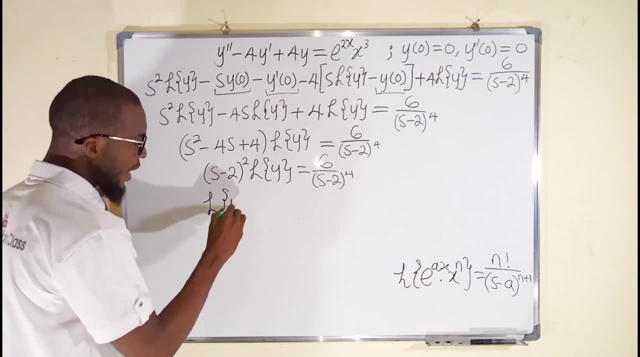 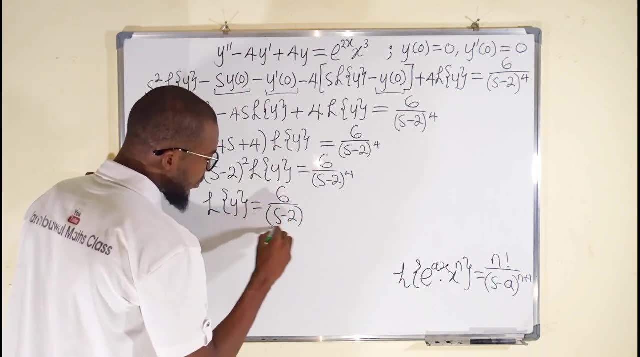 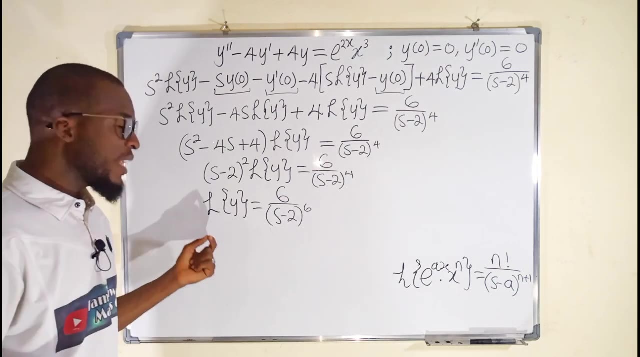 Therefore, to the left hand side, we have the Laplace transform of y Equals 6, divided by s minus 2, to the power of 6.. Because 2 plus 4 is equal to 6.. What do we do next? We can take the inverse Laplace transform of both sides in order to obtain the value of y. 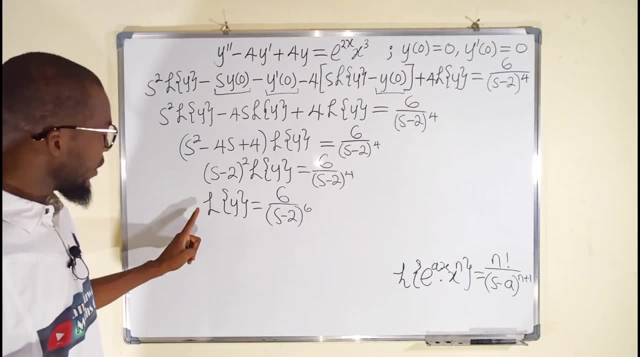 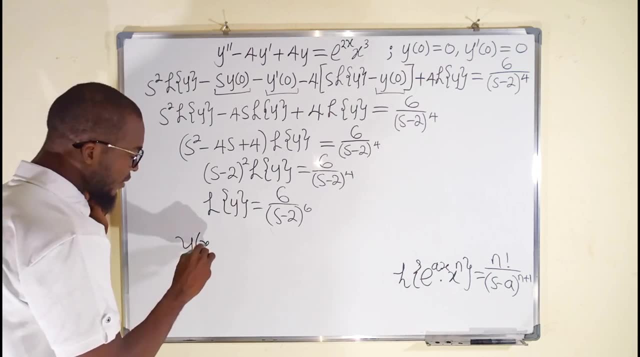 Because inverse Laplace will cancel this Laplace. So, to the left hand side, we have just y, Which is a function of x, And this is equal to the inverse of Laplace. So, to the left hand side, we have just y, Which is a function of x. 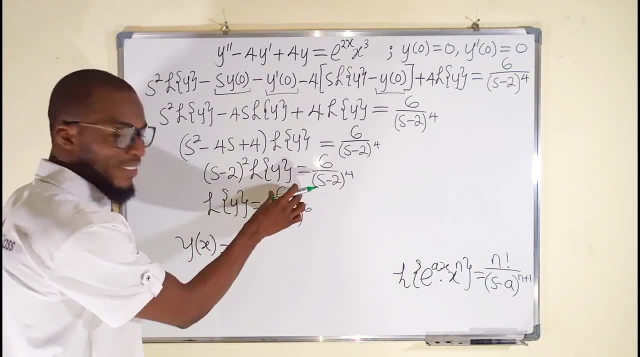 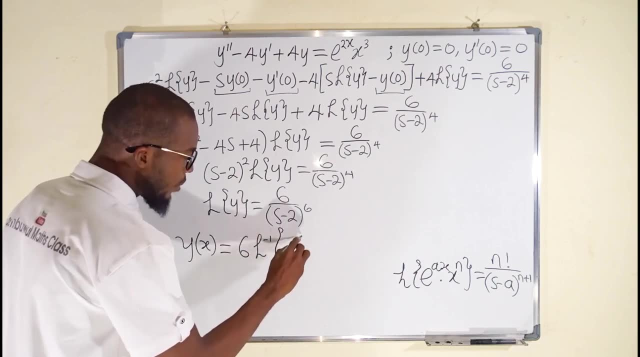 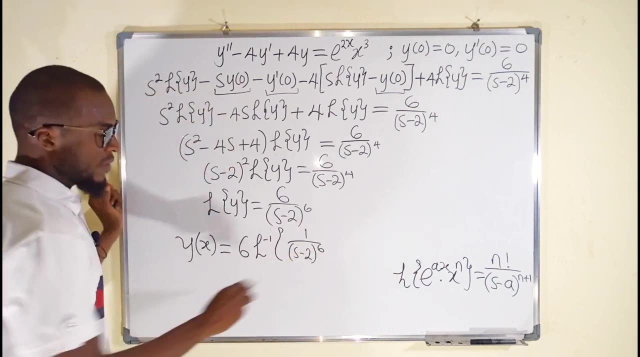 This is equal to the inverse of x. So what we can do next, We can take this Laplace transform inverse Laplace of this, we can factor out six to the top, so we have six: the inverse Laplace transform of one divided by s minus two to the power of six all. 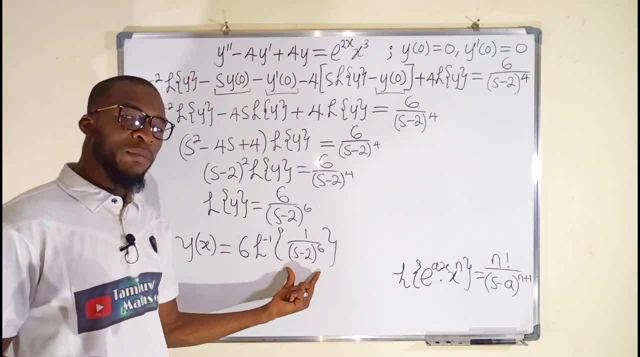 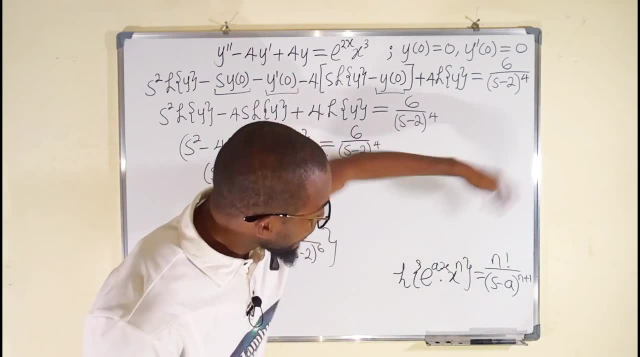 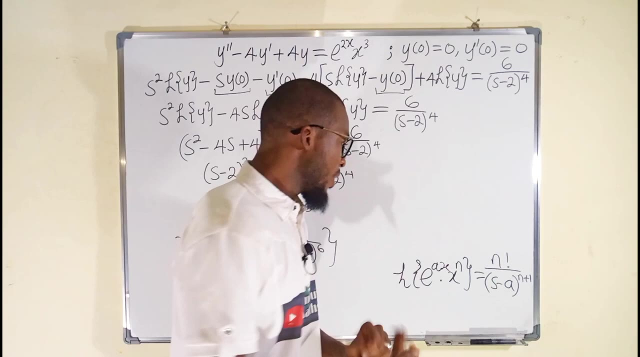 right. how can we find the inverse Laplace of this? remember, if Laplace transform of this is equal to that, if you take the inverse Laplace of both sides. taking the inverse Laplace of this will give us back this function right here, which is a function of X. let's do that. here we have, if we have something. 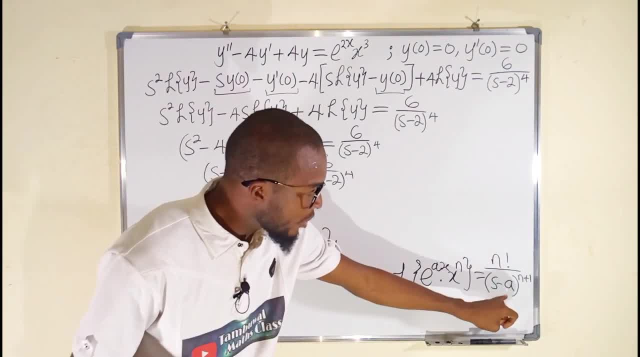 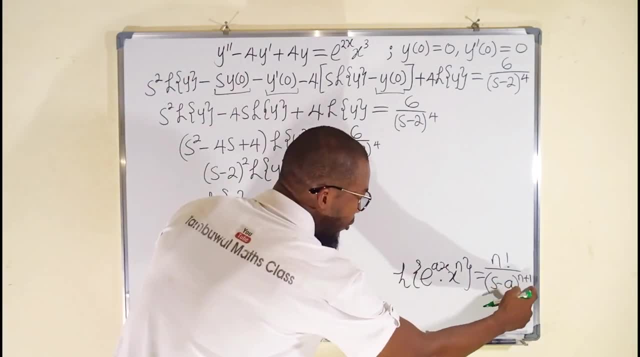 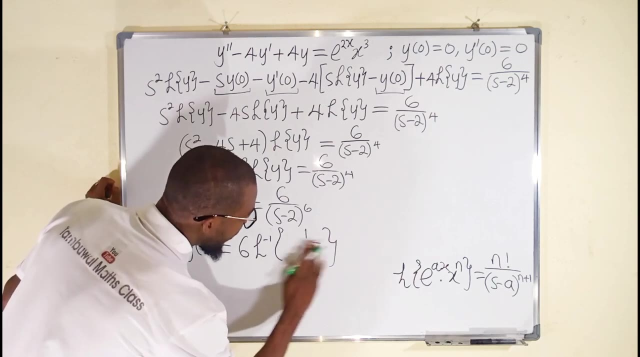 in this form we have n factorial divided by s minus e, raised to the power of n plus one. so we can relate this power of six with n plus one, which is the same thing as five plus one. so we can can write this one as- let me even make it big- 1 divided by s minus 2 to the 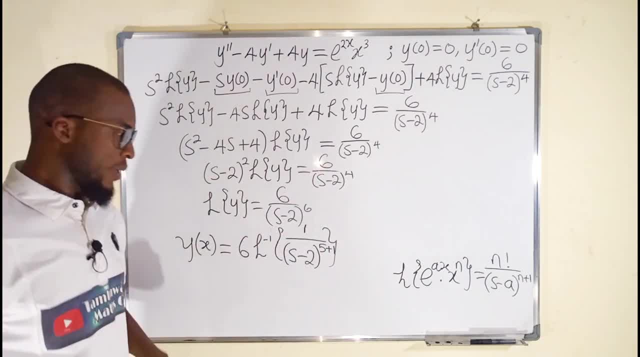 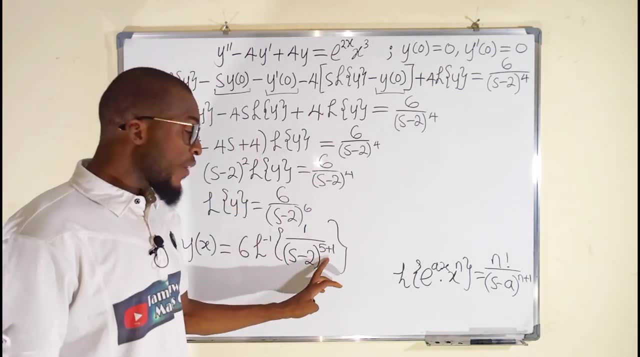 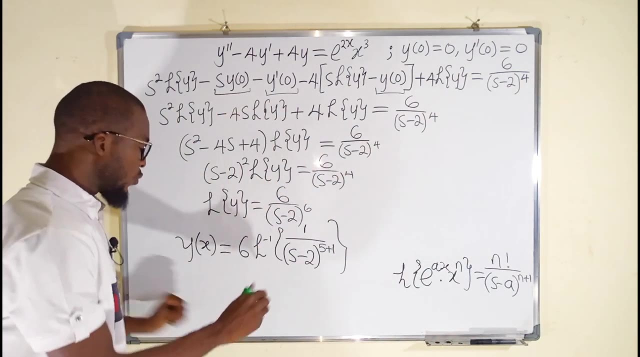 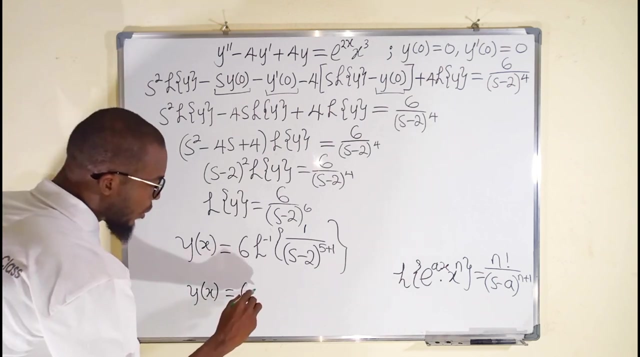 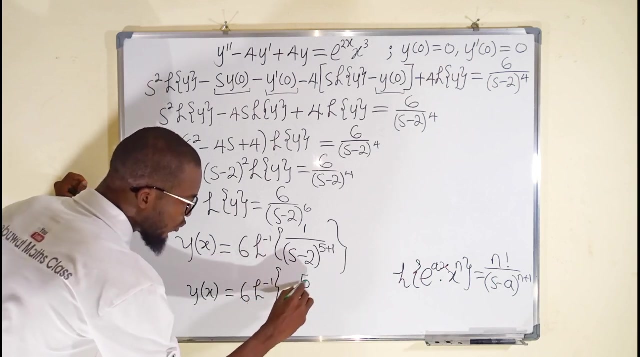 power of 5 plus 1 all right, but having 5 plus 1 here- remember 5 is our n- we have to have 5 factorial to the top. so we can just say that Y of X equals 6 multiplied by the inverse Laplace transform of 5 factorial divided by s.